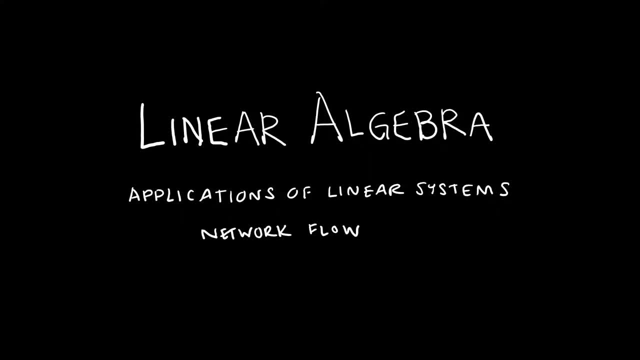 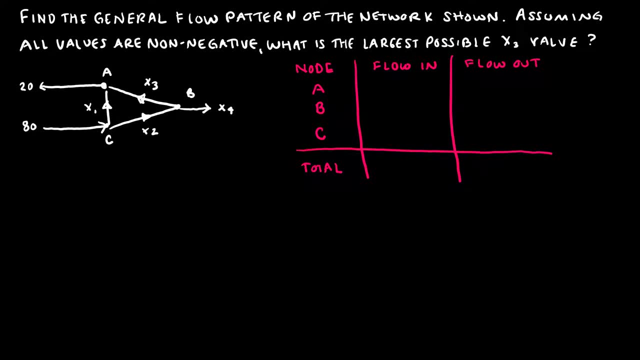 Let's take a look at another application of linear systems in network flow. So where to find the general flow pattern of this network that I've shown? And so in this network, really what we're looking at is each of the nodes A, B and 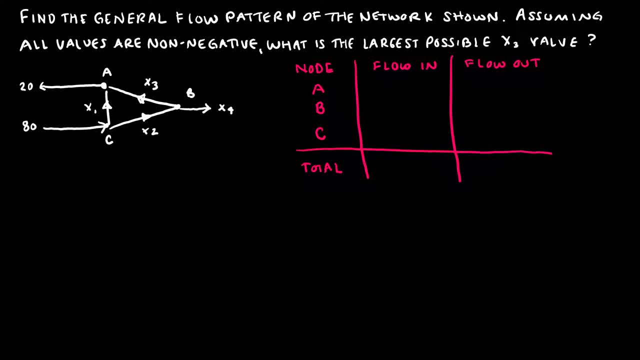 C and we're looking at the flow into those nodes and the flow out of those nodes. So we're going to work through this together and then I'm going to run out of room, I think, on the actual row operations, but we'll do the best that we. 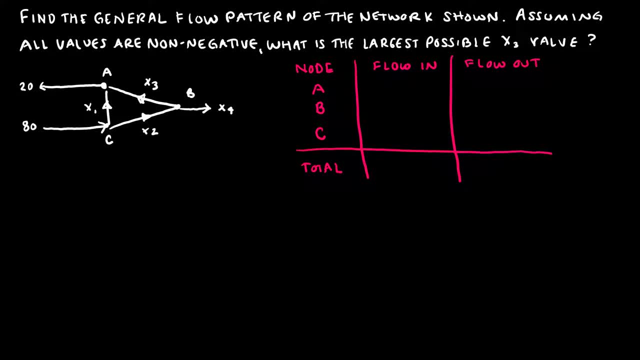 can. So for A, looking at the flow in into A, I have x1, we can see by the little arrow here- and x3, so x1 plus x3 is flowing in and the flowing out of A is 20.. For B, the flow in looks like x2 and only x2.. The flow out looks like both. 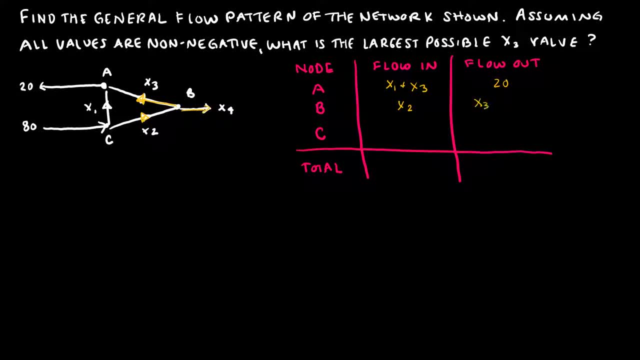 x3 and x2.. So we're going to look at the flow in and the flow out. looks like x1 and x4.. And for C, I have a flow in of 80, right here- and a flow out of both x1. 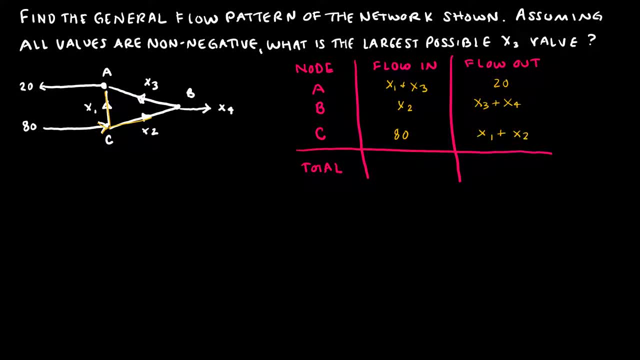 and x2.. So far, so good. And then, of course, I'm going to look at the total, and the total is for the entire network. So flowing into the network is 80, and flowing out of the network is both 20 and x4.. So what I have here is that x1. 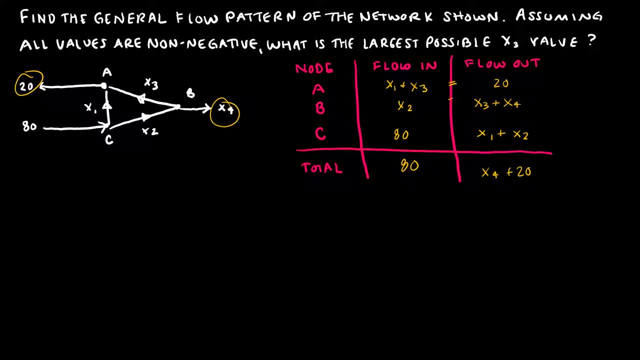 plus x3 equals 20, that x2 equals x3 plus x4, 80 equals x1 plus x2, and 80 equals x4 plus 20.. What I want to do is write those in the correct format so that all of the variables, all of the x's on one side and the constants on the other. 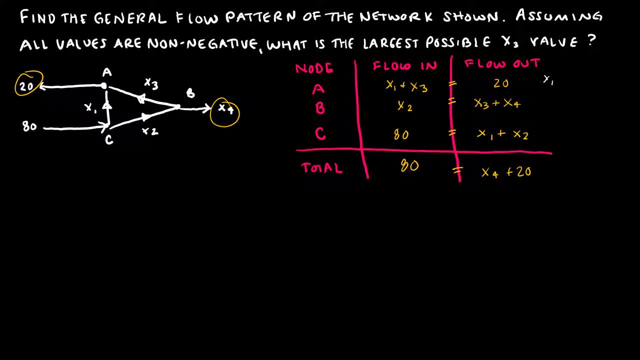 So this is going to turn into: x1 plus x3 is equal to 20.. This one is going to be: x2 minus x3 minus x4 is equal to 0. This is going to be: x1 plus x2 equals negative 80, and this is going to be: x4 equals 60. So from here I'm going to be. 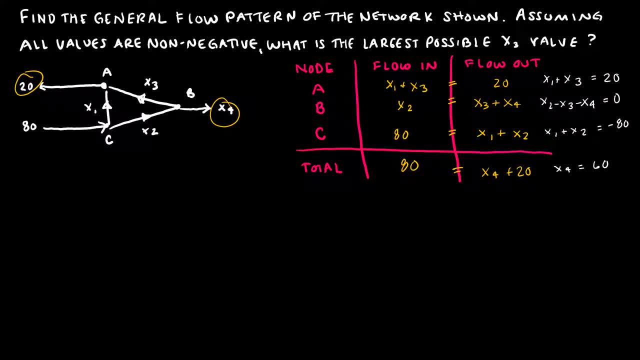 I'm going to- I think I messed up on that- 80. No, x1 plus x2 equals positive 80. Sorry about that. So now I have my system of equations, I can write it in the proper form and I'm 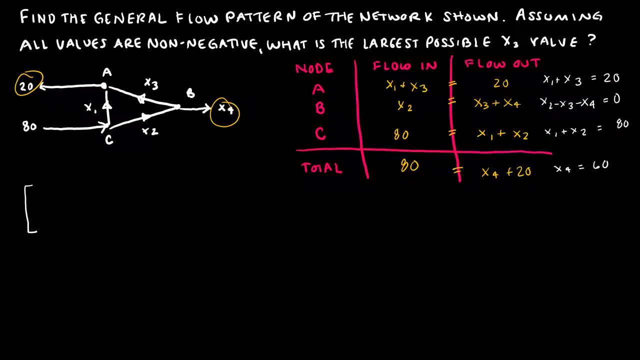 going to try to write this so that I can fit this all on one slide. Otherwise it's going to get a little bit crazy trying to recopy things. So 0 or 1 0, 1 0, 20.. Sorry if that's. 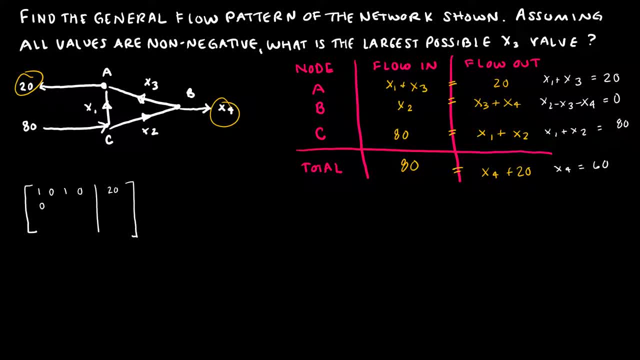 small. Make sure I fit it all in: 0, 1 negative, 1 negative, 1 0, 1, 1 0 0 80 and 0 0 0, 1, 60.. So that's where I stand right now And, just like always, I'm looking for pivots and I'm 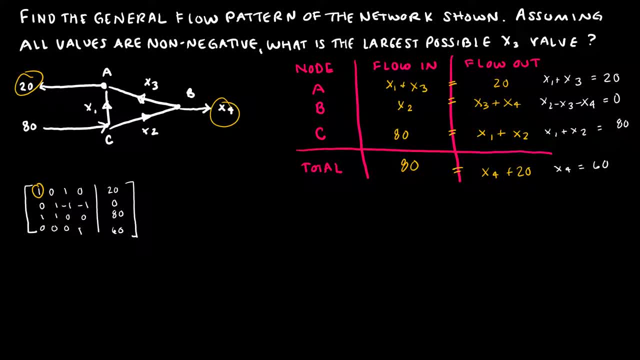 trying to, you know, do the row operation. So I'm going to stick with this guy first for a pivot. Remember, once I have a pivot then everything above or below that needs to be a pivot. So I'm going to stick with this guy first for a pivot And remember: 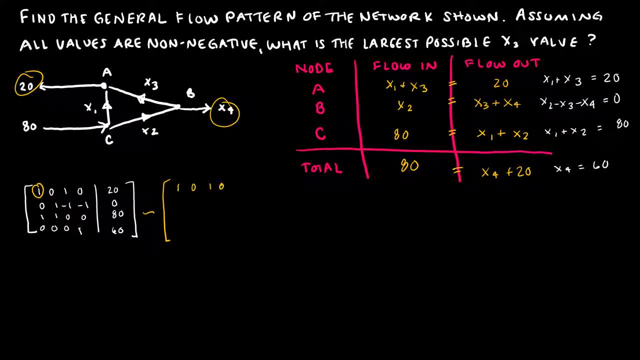 to be a 0.. So this guy is going to remain the same. This guy is already a 0.. Yay, less work for me. I'm just going to subtract the two rows to get that new row. So now I have. 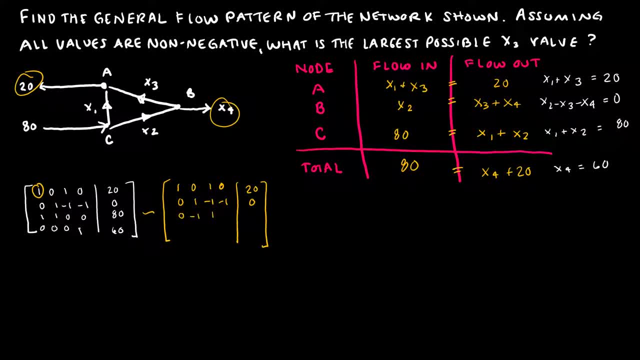 0 negative 1, 1, 0 negative, 60.. And this guy remains the same. So I just took row 1 minus row 3 to be my new row 3.. Um, again, that guy is a pivot. Now I want this guy to be a pivot, So that means anything above. 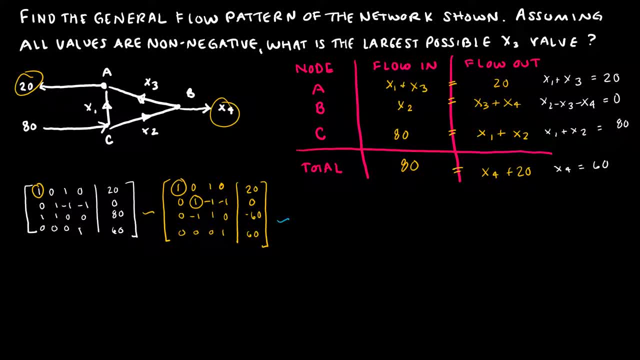 or below that must be a zero. So that's what I'll do next. I'm going to turn this one into a zero. So this guy's going to stay the same. Sorry, I should stop saying this guy. Row one is going. 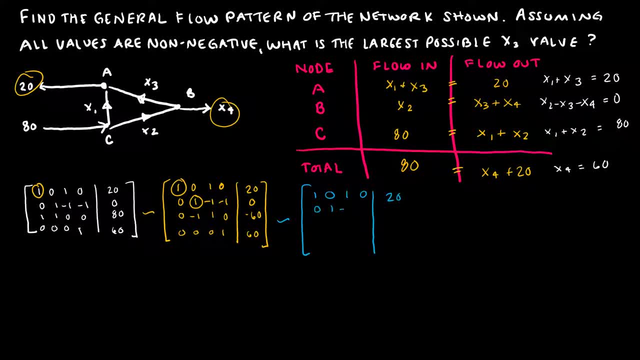 to remain the same, and row two is going to remain the same, And row three? I'm just going to add rows one and row two together to give me zero, zero, zero, negative one, negative 60.. And row four will remain the same From here again. I've got a pivot here. I've got a pivot. 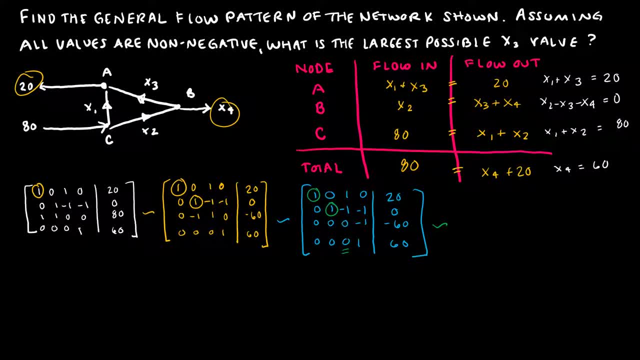 here and it looks like no pivot here in three. So now let's stick with a pivot in four. So really I'm going to do two steps at one. this time I'm going to for row three, I'm going to multiply everything by negative one. So again, nothing's changing here. 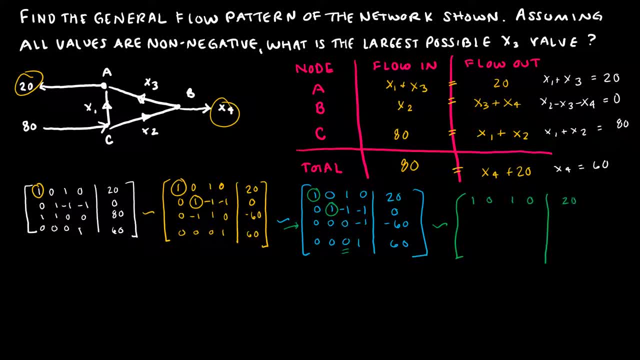 in row one And in row two, nothing's changing. Lost my place for a second Row three. I'm just going to take everything times negative one And row four. I'm going to add rows three and four together to get zero. 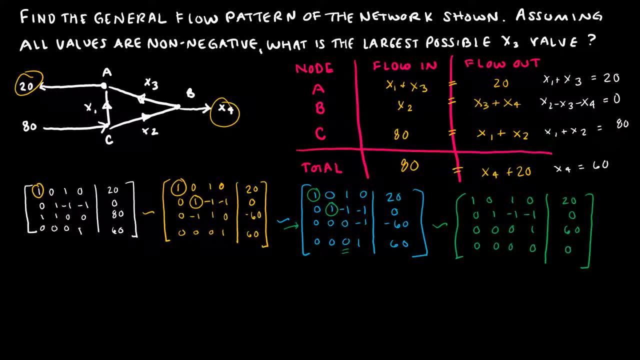 zero, zero, zero, zero. So obviously we can see that row three. I'm sorry that x three is a free variable, But now I have to continue because I need to. I have a pivot here. So I have a pivot here and all the 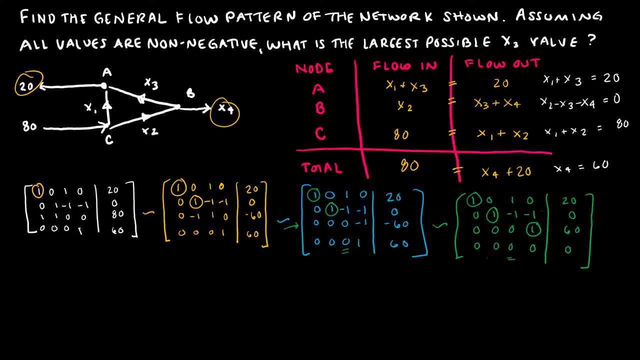 zeros are good- And I have a pivot here- and all the zeros are good, But obviously we have a problem right here at negative one. So that's my next operation is, I need to essentially just add rows two and three together And that's going to give me a final. 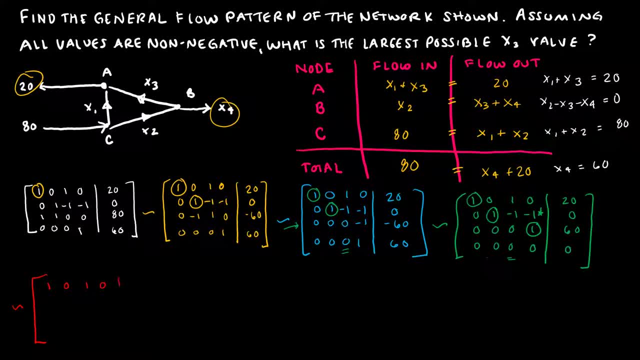 matrix of one zero, one zero, 20, zero, one negative, one zero, 60, zero, zero, zero, zero. just kidding, Got a little zero happy there. One, 60 and zero, zero, zero, zero, zero, And that's. 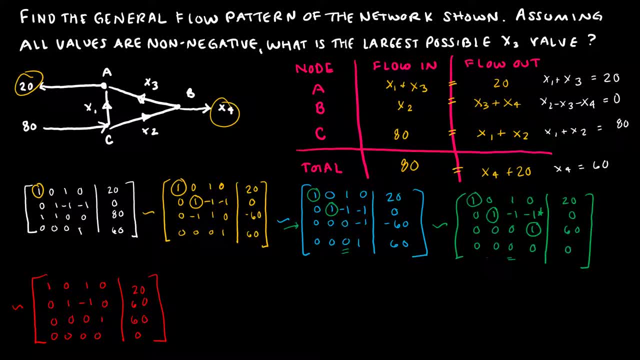 what we have. So what are we going to do from here? Essentially, I want the general flow pattern, which is the same as me saying what's the general solution. So the general solution is that x one is equal to 20 minus x two. 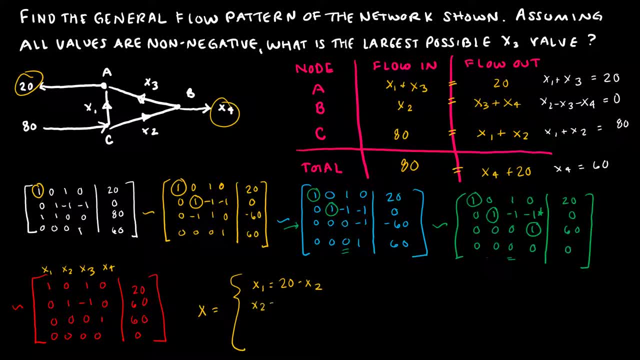 And that x two is equal to 60 plus x three And that x three is free And that x four is equal to 60. So that answers the first part of this question. What's the general flow pattern of the negative network? That is the general flow pattern. Then it says: assuming all values are non negative. 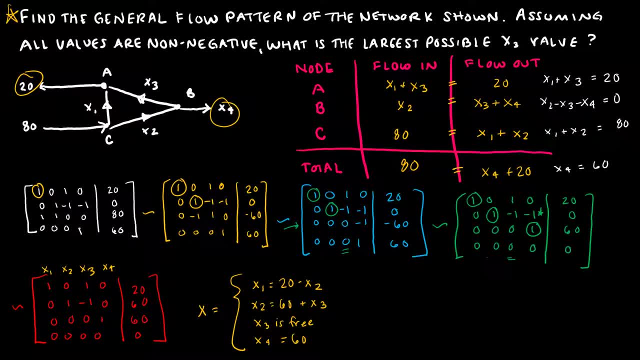 what's the largest possible x three value? So really, the largest possible x. I did something wrong, I'm sorry. This is x three, 20 minus x three. That was important because obviously now the largest possible x three value is 20.. Because 20 minus 20 is minus 20.. And we've got the largest.